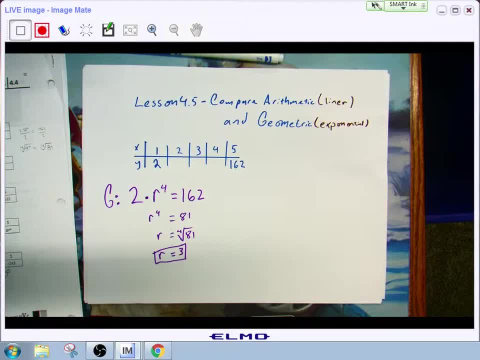 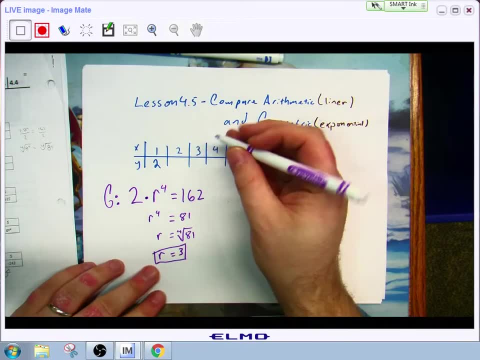 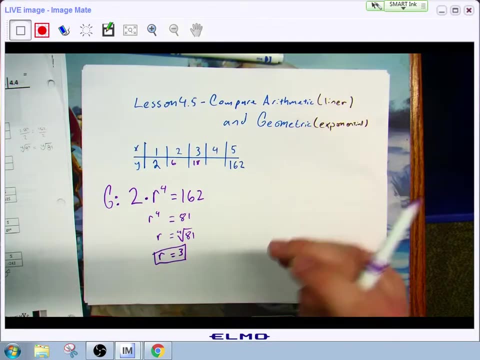 So I know that my ratio is 3, that means I'm multiplying by 3 each step. So when I multiply by 3 each step, 2 times 3 is 6, times 3 is 18, times 3 is 54.. 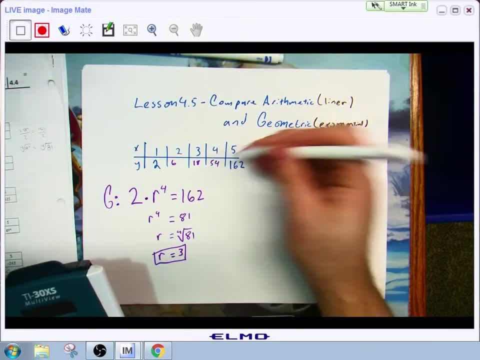 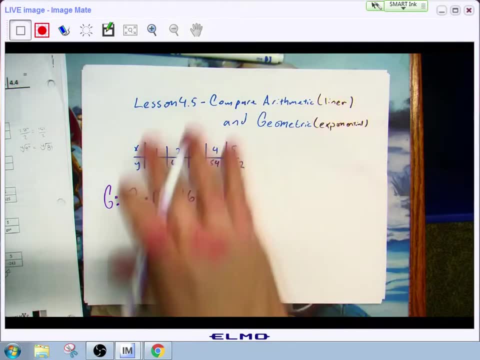 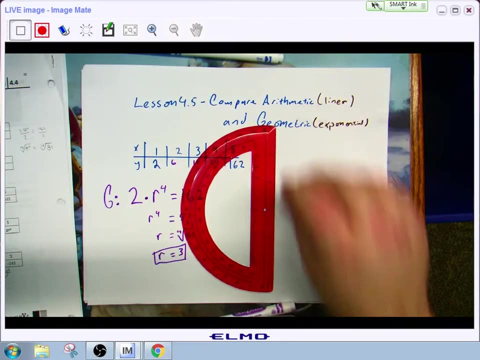 Is that right? 54, 54 times 3 is 162.. And so I'm able to construct that by figuring out that ratio. And, in fact, if I were to graph this, which I will right now, let's look to see what it looks like. 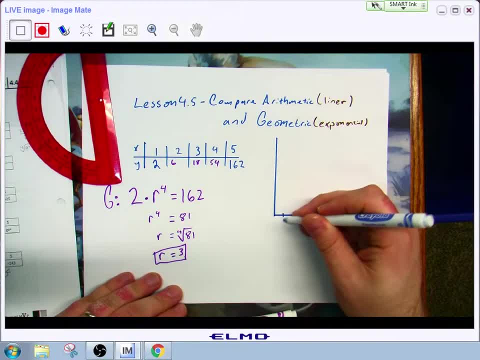 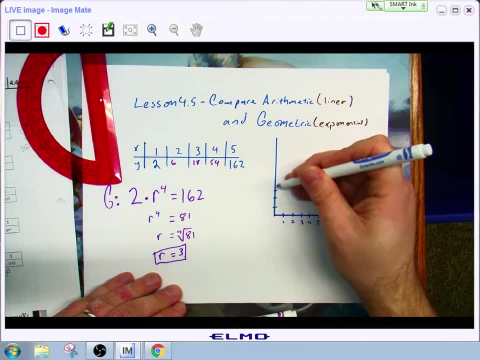 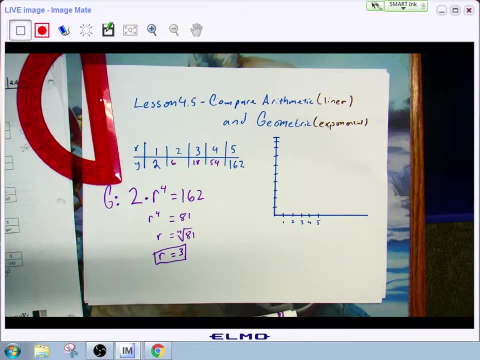 If I were to graph this. so I have 1,, 2, 3.. 1,, 2,, 3,, 4, 5.. One thing I want to draw your attention to is the idea of scale. Yeah, that's it. 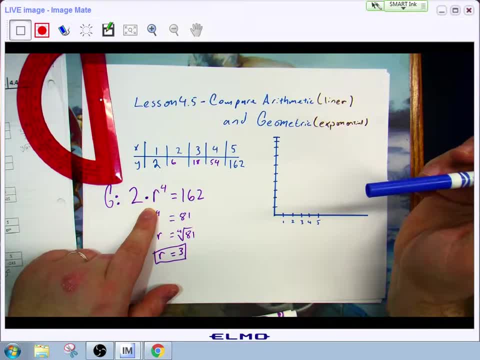 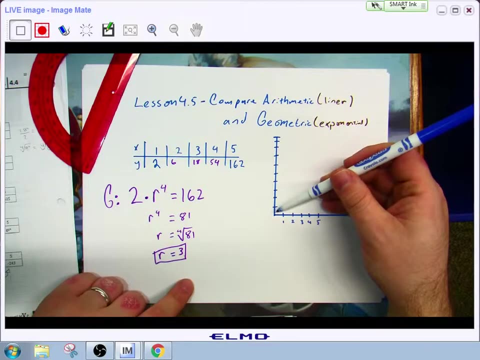 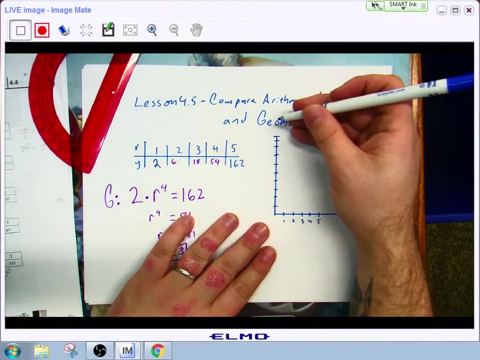 2 to the 4th power. I'll have to look at it later, just to double check it. Okay, Um, when we're looking at this and I'm asking you to graph this clearly, we do not have room to make 162 hash marks. 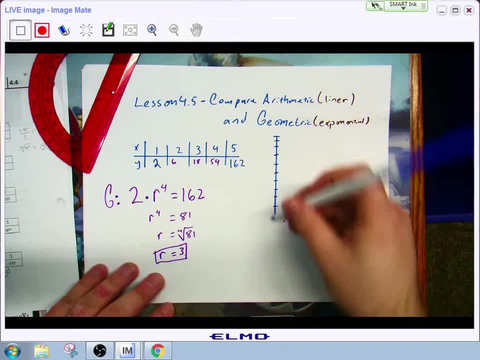 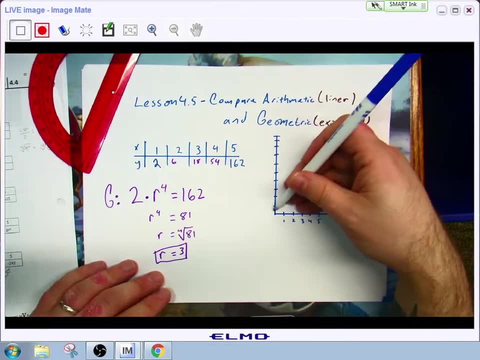 So we have to do something called scaling. okay, We have to scale what each of these lines will be, And if I have to get all the way up here to be 162,, that means each of these lines will be counted for more than 1.. 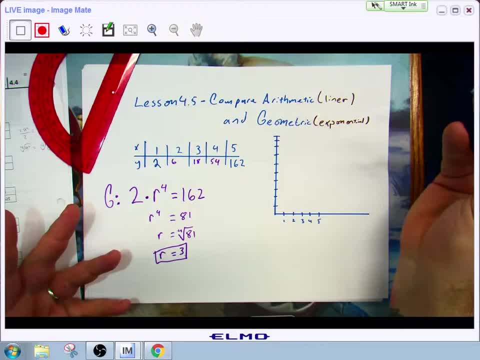 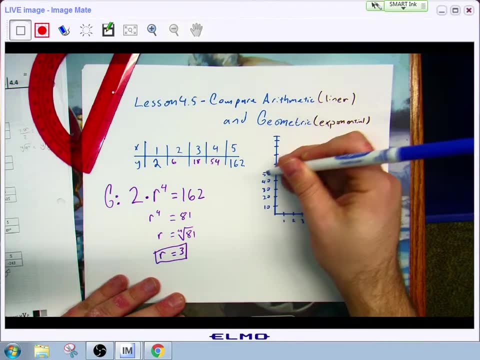 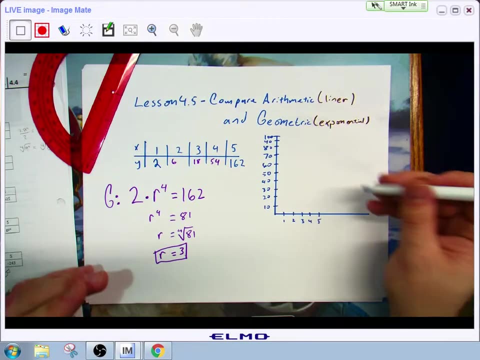 Okay, I'm just going to keep going. Yes, then our appropriate scale would be about 10.. So this is going to be 10,, 14,, 13.. 100.. I'm still going to be a little bit short, but it will be enough for me to at least have a good one. 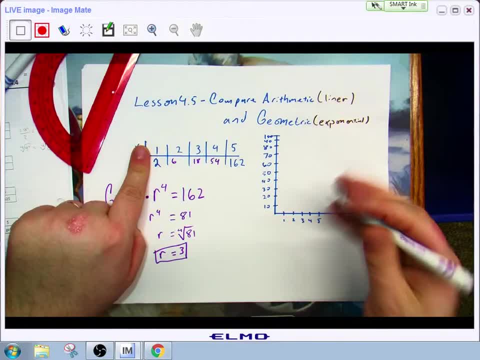 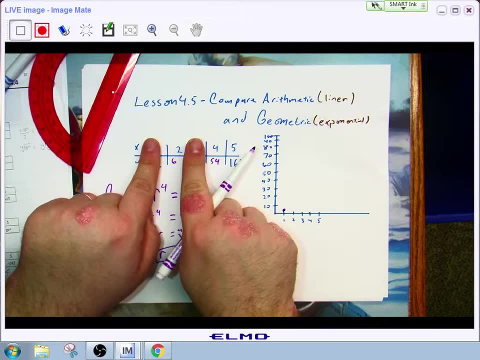 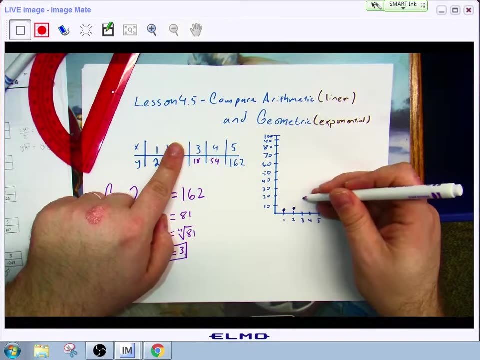 Now I'm going to plot my points. I know that the point 1, 2 is a point That's going to be right there And I've been doing this in the notes Here: 2, 6.. 3,, 8, 10.. 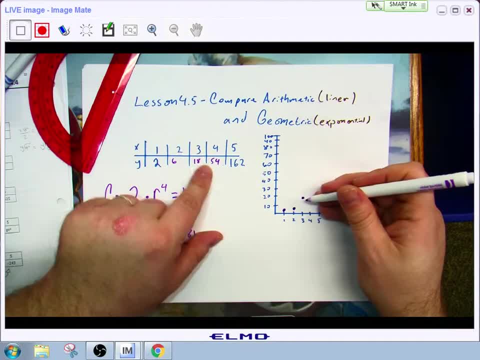 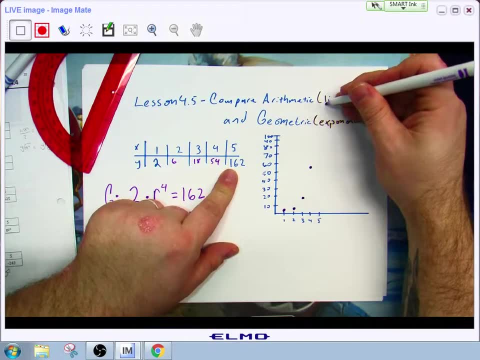 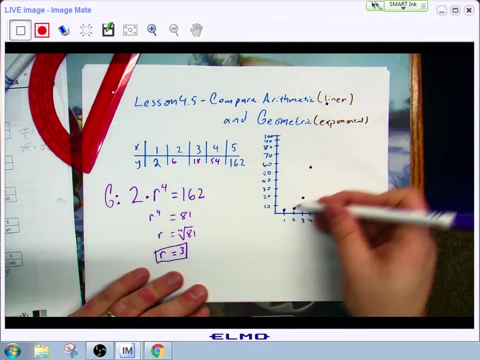 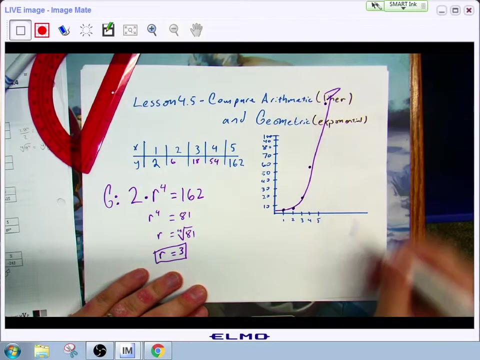 That's going to be almost 20.. Almost 54. And 562.. And you can see, when I do this, what I end up with is I end up with a curved graph, I end up with a line And it's an upward flat graph. 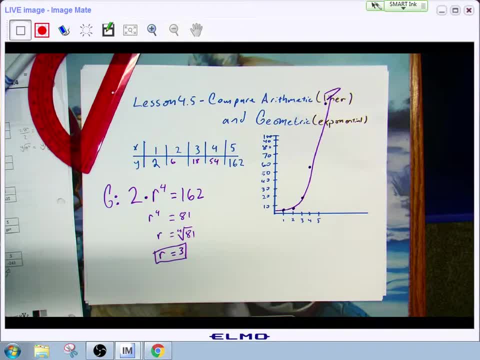 Easy enough. Well, let's assume now Does everyone have this in their notes? I don't want to move ahead until we're set to go. Give me a thumbs up if you're a little bit more excited, A little bit more time. 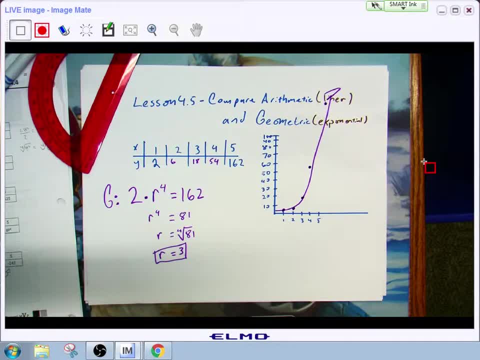 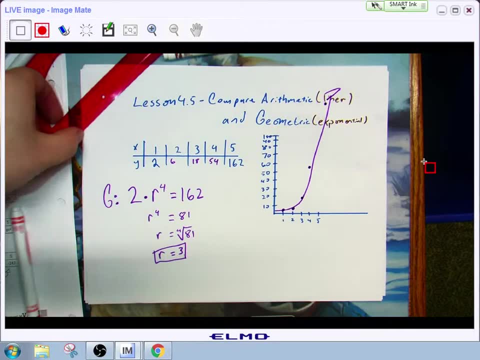 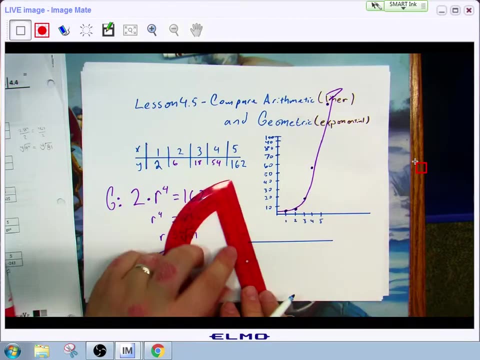 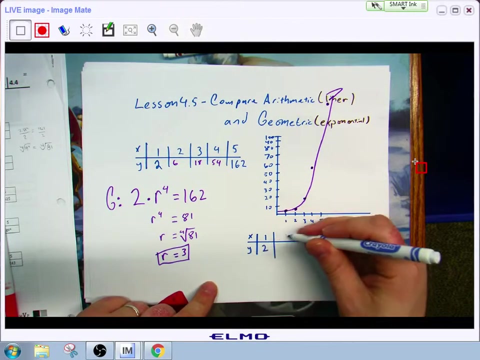 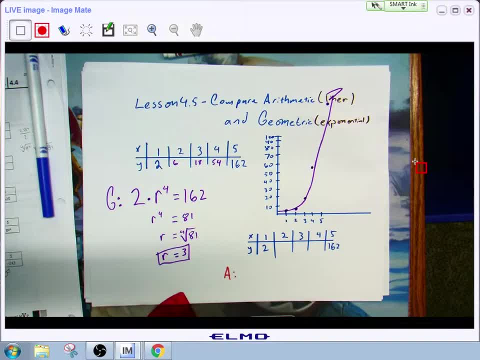 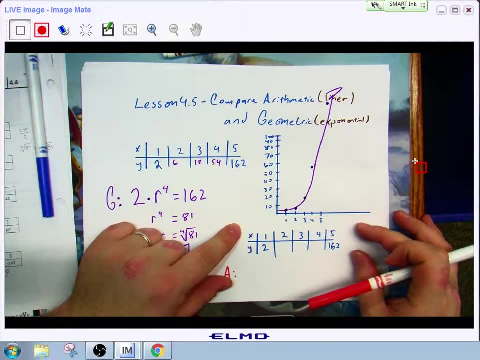 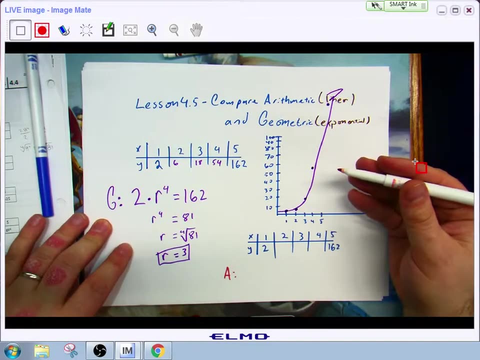 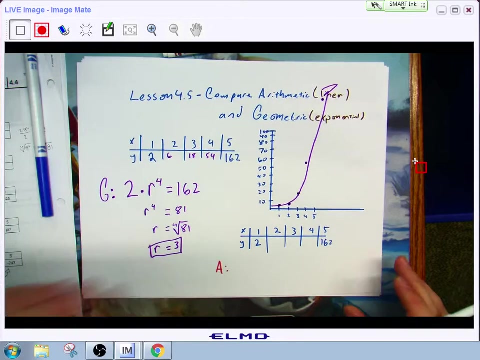 this time, what I want to do is, let's say, I was given this exact same form and these exact same lines here as I was given up here, but this time, instead of being asked to find a geometric pattern, I want to find the arithmetic pattern. if this is my start point, that was my end point. what does that look like in the form of an arithmetic pattern? let's give that a try. 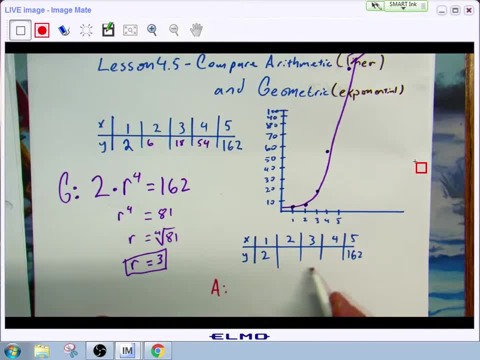 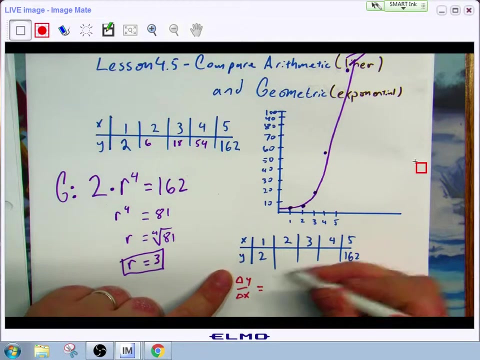 this time what's happening is I'm adding by a certain amount, right. this time, instead of multiplying, I'm adding. but one of the easiest things about this: we can do this just as a slope formula, right, because I can do my change in y over my change in x and figure out my slope. so to do that, I have my y2, which is 162,, subtract my y1, which is 2, and then I take my x2,.